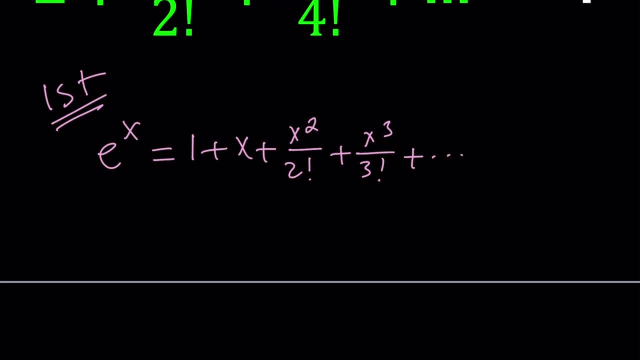 can do it, and I believe we've done this in another video. If I can find that video, I'll try to link it. But if you set f of x equal to e to the power x, and then just think about writing it as an infinite polynomial, such as a sub 0 plus a sub 1 x plus a sub 2 x, 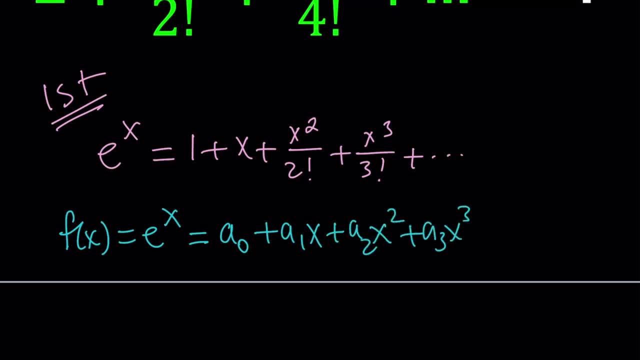 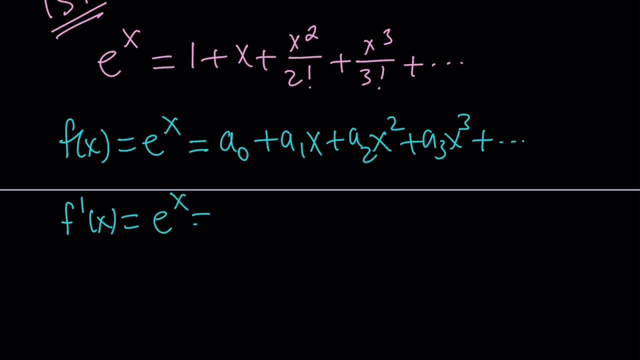 x squared, plus a sub 3, x cubed, and then so on and so forth, And then you're going to differentiate this function a few times. Every time you're going to get e to the x, but on the right hand side, since we have an infinite polynomial, the derivative is going to be a. 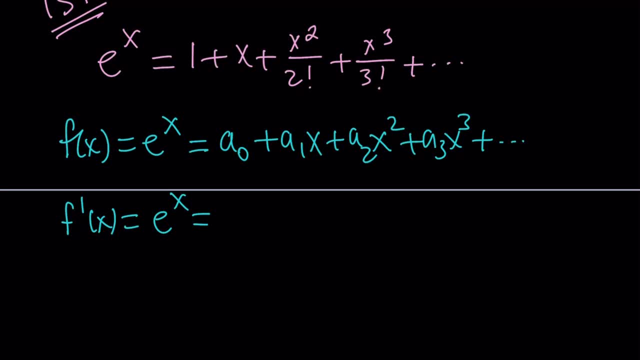 little different, even though it's the same thing. Anyways, the derivative of a sub 0 is 0 because it's a constant, and then this is going to become a sub 1.. This is going to be 2 a sub 2 x, and it's going to be 3 a sub 3 x squared. 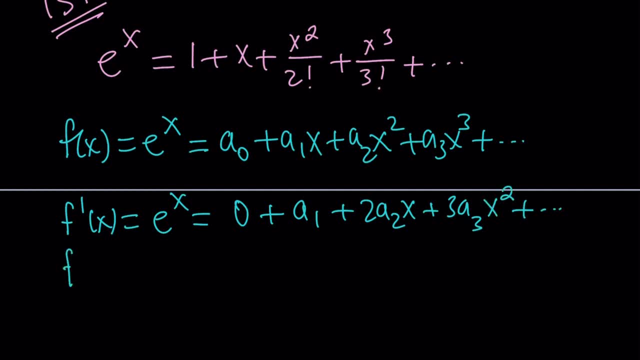 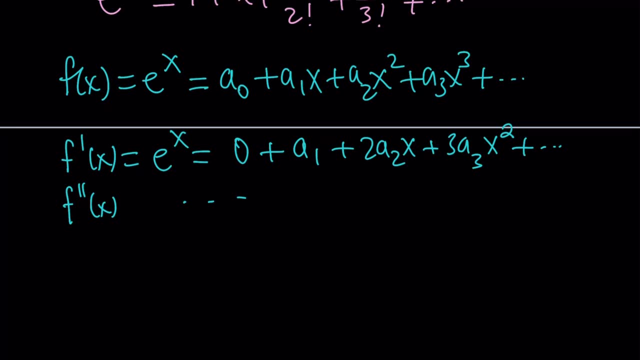 And so on and so forth. And then we're going to differentiate it again, so on and so forth. So, after all these derivatives or differentials, you're going to replace x with 0. So you're going to evaluate f of 0, f prime at 0, f double prime at 0, so on and so forth, And then set: 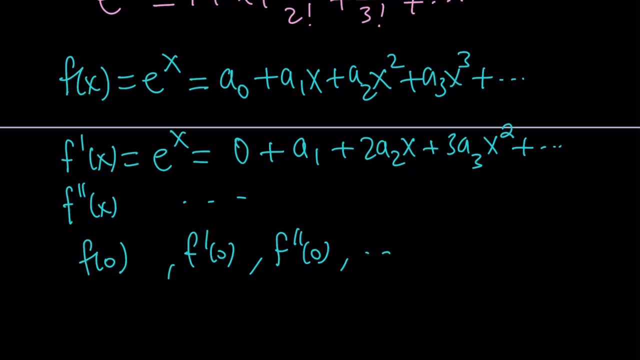 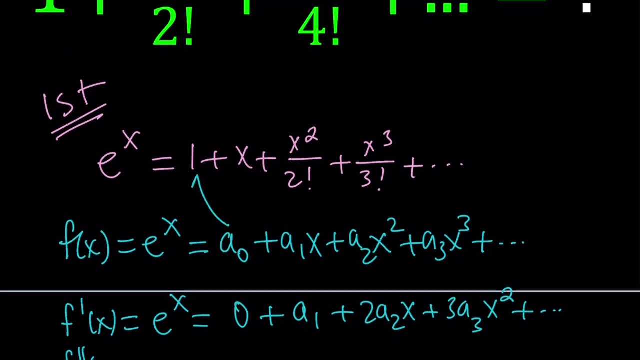 it equal to each other. And then, from there, you're going to be able to evaluate a sub 0, a sub 1.. And you're going to realize that a sub 0 is 1, a sub 1 is 1, a sub 2 is 1.. And 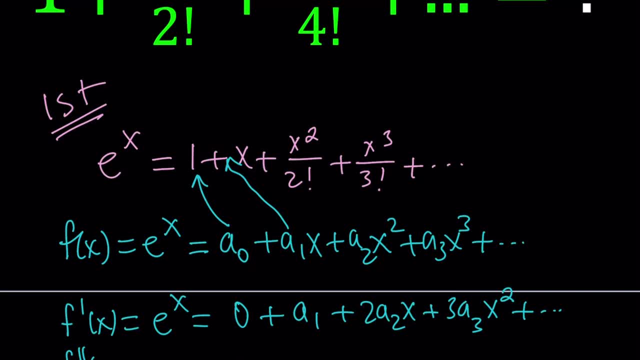 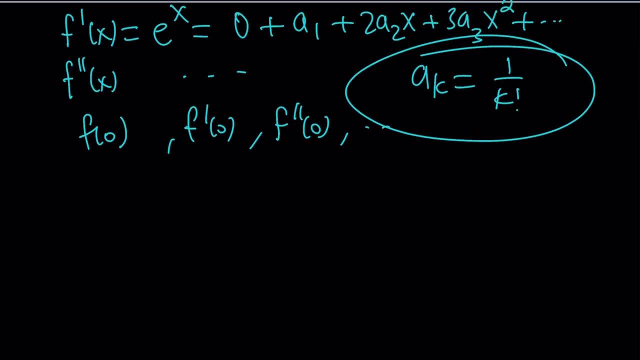 so on and so forth, So that a sub k is always 1 over k. factorial. Make sense? That's what's going to happen. To keep a long story short, we have the following: e to the x equals 1 plus x plus x squared divided by 2. factorial plus x cubed over 3. factorial plus x to the. 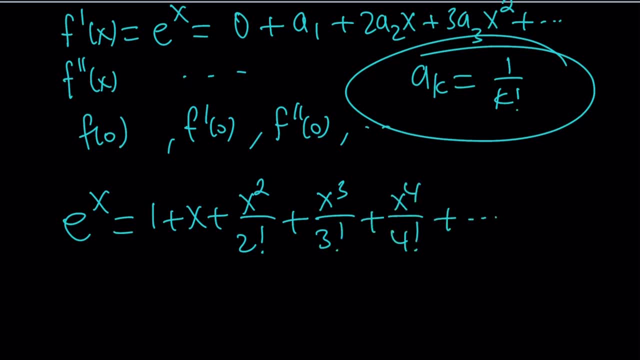 fourth, over 4, factorial, so on and so forth. Now I want to get the sum of the reciprocals of even factorial. I need to get rid of some terms, Right? What are they? I need to get rid of this. I need. 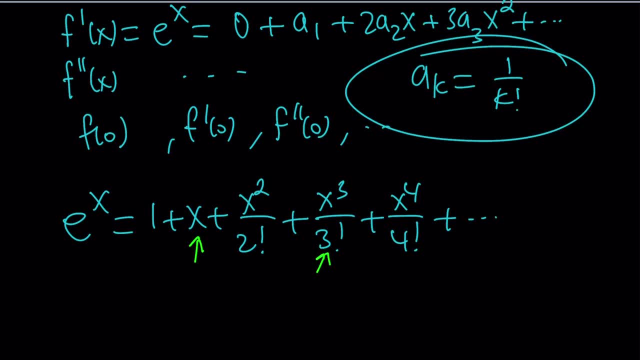 to get rid of this, And so on and so forth. But how do you achieve that Right? Well, here's the thing: You can always negate those terms because of the odd powers. So let's go ahead and replace x with negative x on both sides. That's going to give us the following 1. 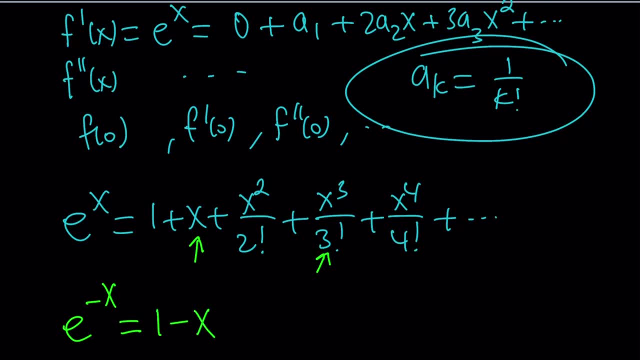 minus x. Right, Because x is being replaced with negative x Plus negative x squared is the same as x squared, So it's not going to change. And then the x cubed: If you cube negative x, you're going to get the opposite of x cubed, which is going. 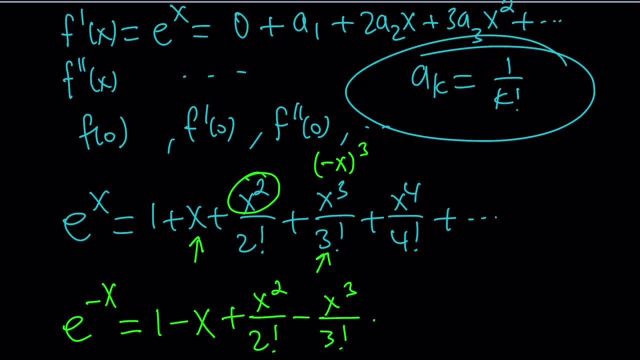 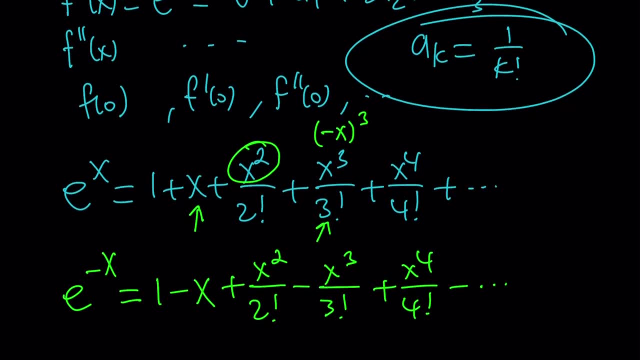 to give you a minus sign, So on and so forth. So you're basically going to get all the odd factorials with a minus sign Right, And of course the next one is odd too. And then here's what we want. We want to get rid of the odds, So let's go ahead and add these up. Ok, That's. 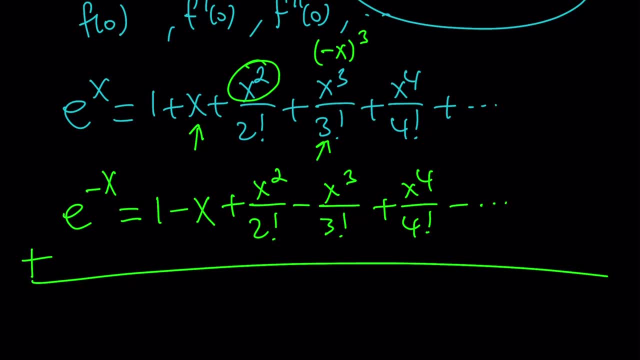 just going to give us another Taylor, Taylor expansion or Taylor series, which is for e to the x plus e to the negative x, And of course that's going to be 1 plus 1.. These terms are going to cancel out These terms. 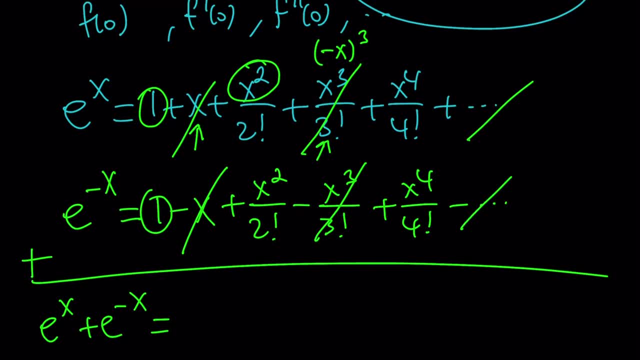 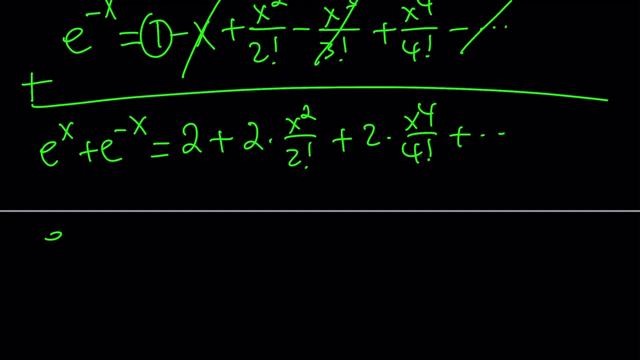 are going to cancel out. All the odds are going to cancel out. We're going to end up with 2 plus 2 times x squared over 2 factorial. Don't simplify that yet. 2 times x to the 4th over 4 factorial. So on and so forth. Notice that we can take out a 2. Right, And when we do, we're going to. 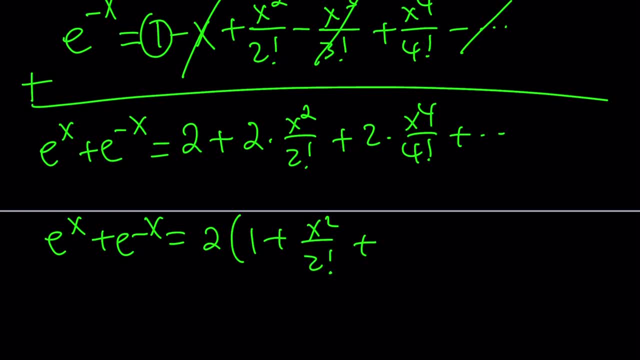 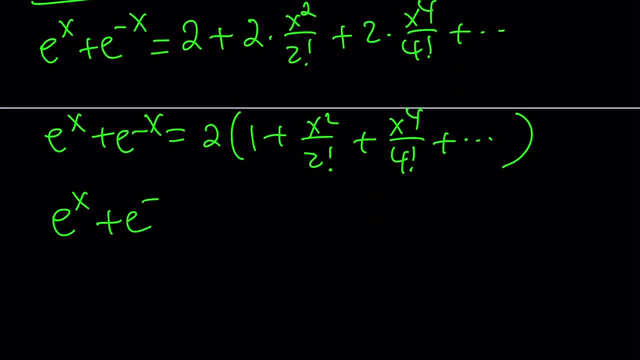 get 1 plus x squared over 2. factorial plus x to the 4th over 4. factorial Dot dot dot. Now here's what we want. We want to divide both sides by 2, because that's going to give us, that's going to bring us even closer to the. 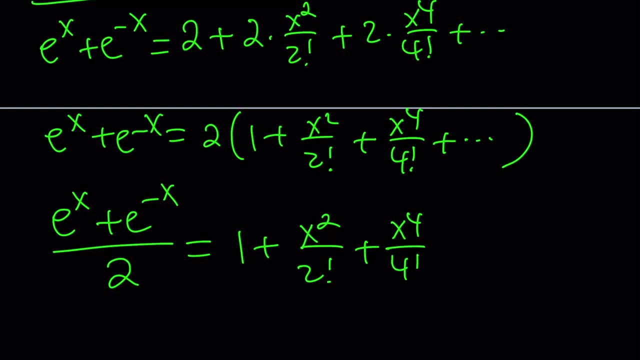 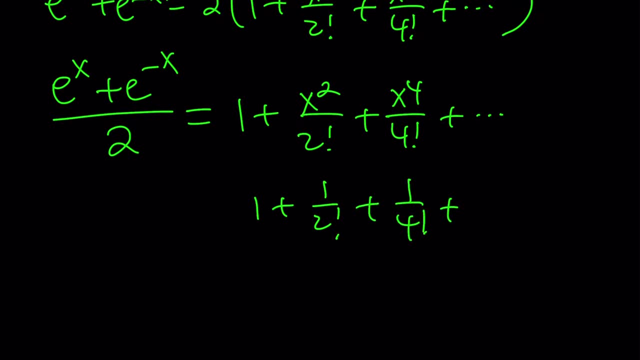 sum that we're trying to evaluate And notice that our sum is just 1 plus 1 over 2 factorial, plus 1 over 4 factorial plus 1 over 6 factorial, So on and so forth. So all we have to do is replace x with 1 and we're good to go. 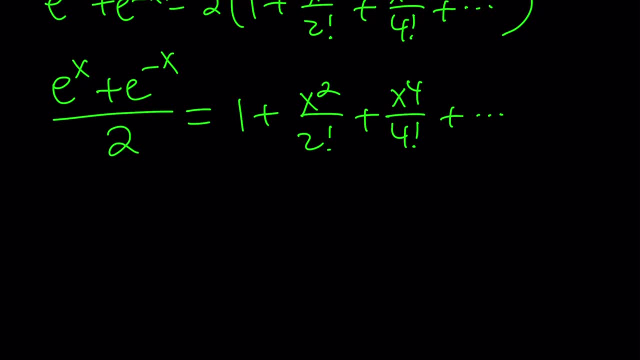 Make sense. So we're going to go ahead and replace x with 1 on both sides, And then it's going to be e plus e to the negative 1, or just we can write it as 1 over e. I guess, divided by 2 equals 1 plus 1 over 2 factorial plus 1 over 4 factorial plus 1 over 6 factorial. blah, blah blah. That's what we want. 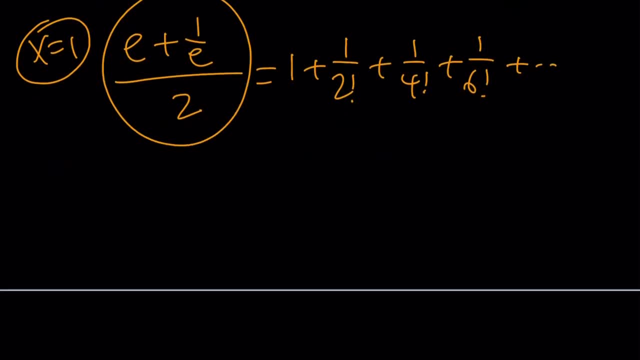 And so this is the answer, And if you simplify it, you're going to get e squared plus 1 divided by 2e, as our answer Make sense. Okay, great, Let's go ahead and talk about the second method. Now, obviously, the second method is a: 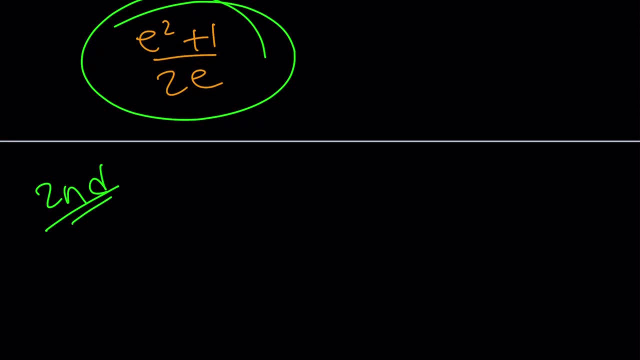 little different They are. they are related but it kind of uses a different idea And of course we're going to take advantage of Taylor expansions or Taylor series again. So consider the series for cosine. that is 1 minus x squared over 2. factorial plus x to the fourth over 4. factorial minus x to the sixth over 6. 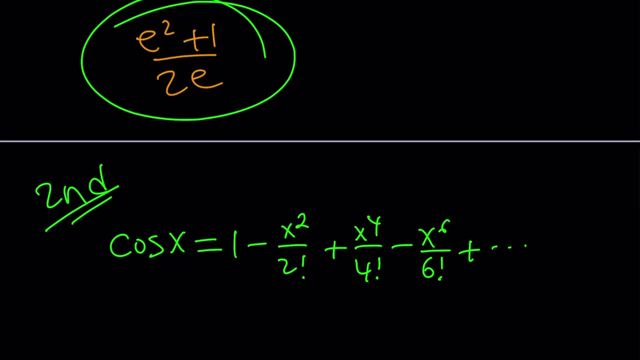 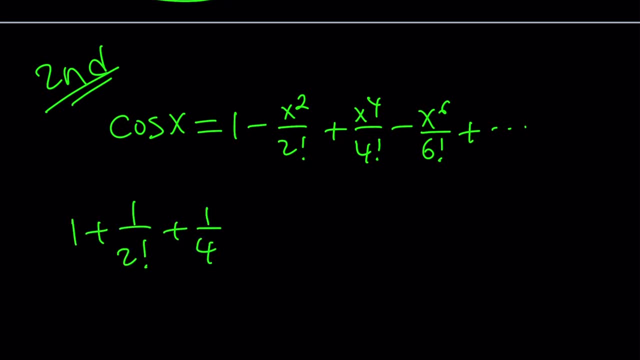 factorial plus dot, dot dot. It's kind of like an alternating series. the sines will alternate And remember, we're looking for this right. So we actually don't want any negatives. So the million-dollar question is: can we fix the negatives? And the answer is: 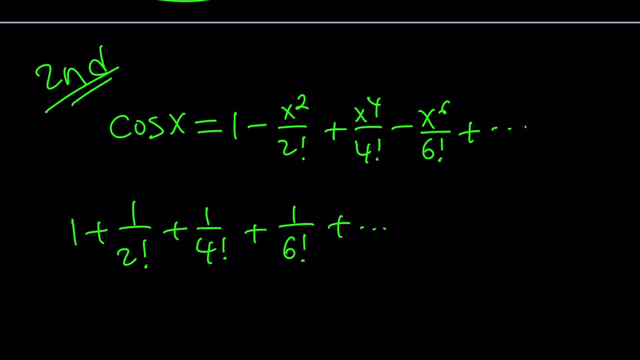 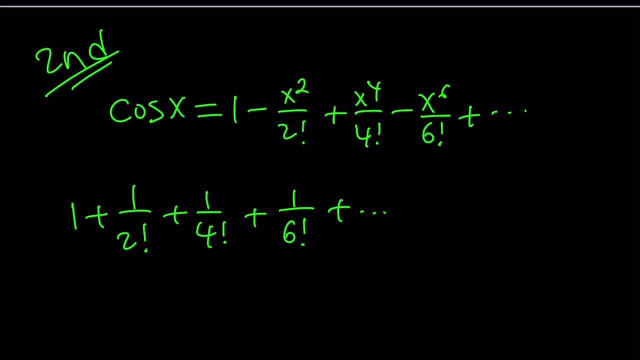 of course. That's what math is for: right- To fix all the problems. So here's what we can do. We can go ahead and replace x with something that is almost magical, or maybe I should say mathemagical, so that every negative turns into a positive. So here's what you need to consider. 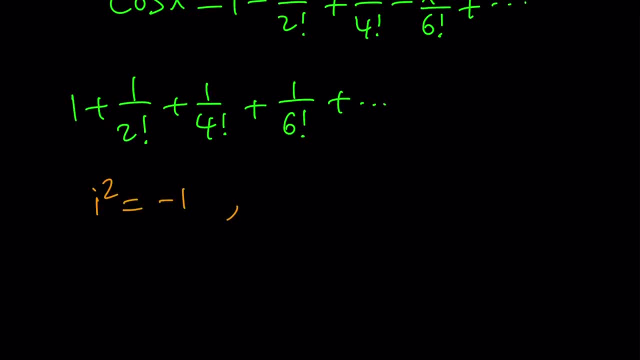 Note that i squared is negative 1, and i to the fourth power is positive 1.. In general, i to the power 4n is 1, and i to the power 4n plus 2 is negative 1, if n is an integer. 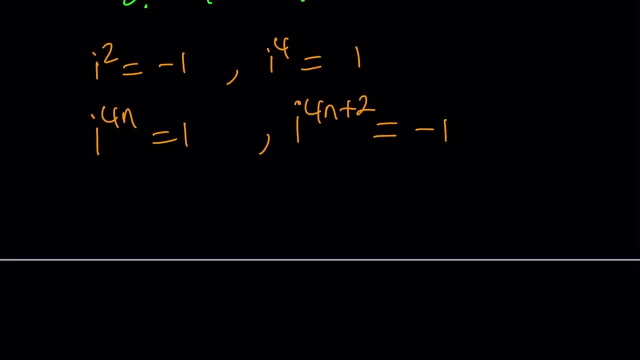 a positive integer, I think right, Or a non-negative integer. Anyways, this is nice because we can just plug in the negative. So we can plug in the negative, So we can plug in the i, So cosine, i is going to be remember the expression for cosine, Let me just copy that here. 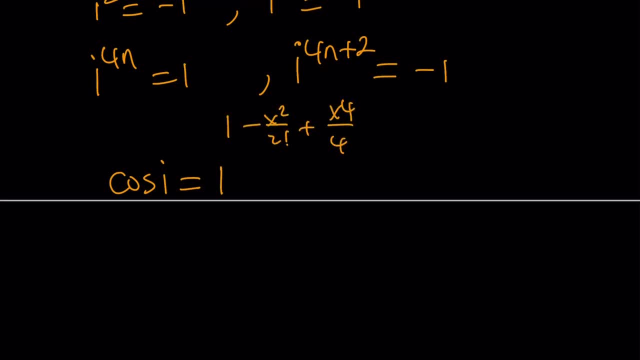 so you get to see what I'm doing again. This is the cosine. And then if you go ahead and replace x with i- this is cosine of x- you're going to get 1 minus i, squared over, 2 factorial plus i to the. 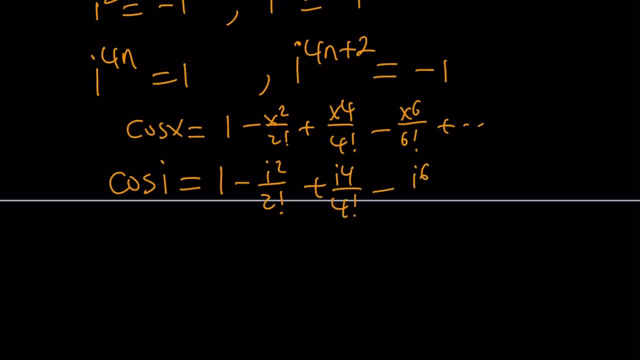 fourth over 4 factorial, minus i to the 6 over 6 factorial. And yes, the mathemagic happens and i squared is negative 1.. So you get 1, plus 1 over 2 factorial, plus 1 over 4 factorial, plus 1 over 6 factorial, and so on and so forth. 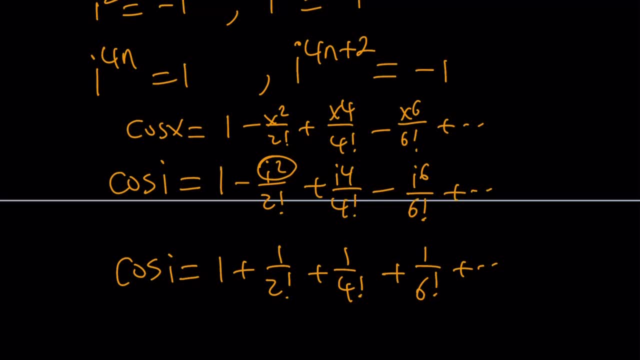 And that's what you want. But what is cosine i? I think we've done that in another video too. Again, if I remember, I'll try to link it. But to keep a long story short, I think we also talked about it.